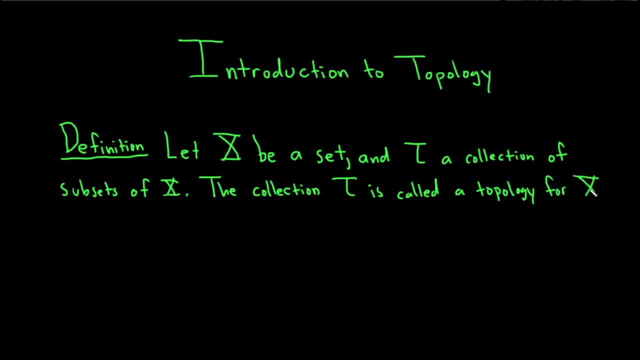 Then we've got this expression that says: provided tau satisfies the following conditions. So provided tau satisfies the following- You can call them axioms or conditions or criteria. I'll just say: satisfy the following satisfies the following, So one. so the first condition is that the empty set and capital X. 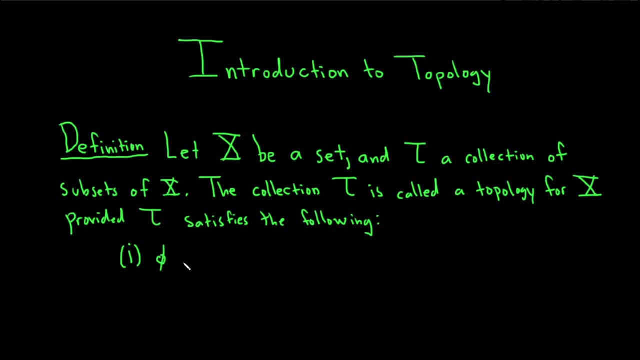 are elements of tau. So the empty set and capital X are elements of tau. So that is the first condition that we require. The second condition is that if you have two elements in tau, the intersection of those elements is also in tau. Now some textbooks and some authors require that you have a finite set, but you can easily show 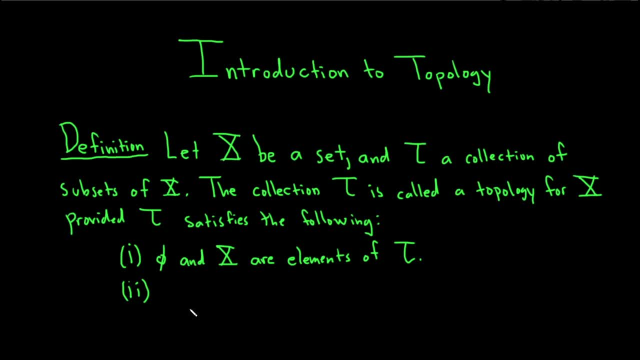 that you have a finite set. So if you have a finite set you can easily show that you have a. that will follow from our definition using mathematical induction. So let's just stick with two. So if say, O sub 1 is in tau and O sub 2 is in tau, then O sub 1 intersected. 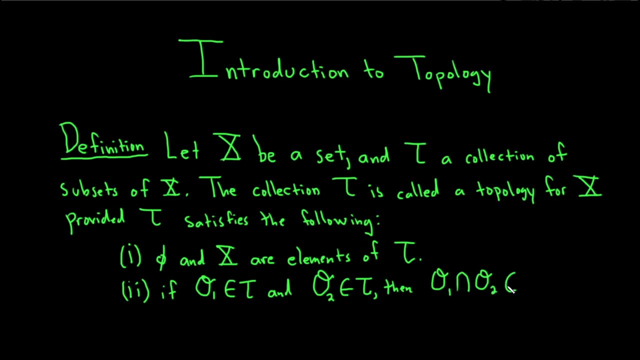 with O sub 2 is also an element of tau, Really really nice. And the third condition is that if say we have some arbitrary collection O sub i and this is a subset of tau, So each of these O sub i's is a subset of tau. So each of these O sub i's is a subset of tau. 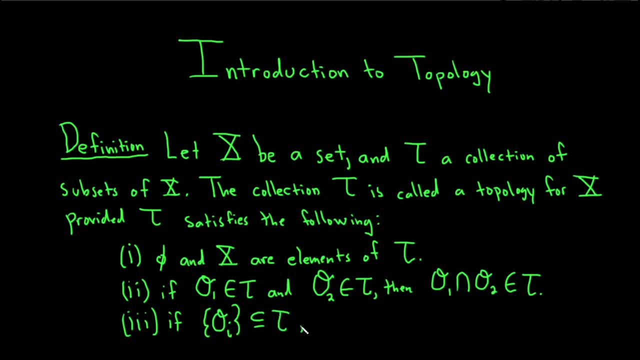 O sub i's is an element of tau, Then if we take the union of the O sub i's, then this is also in tau. And this is just any union. It's not necessarily finite. So it could be just any arbitrary collection. It doesn't have to be finite. 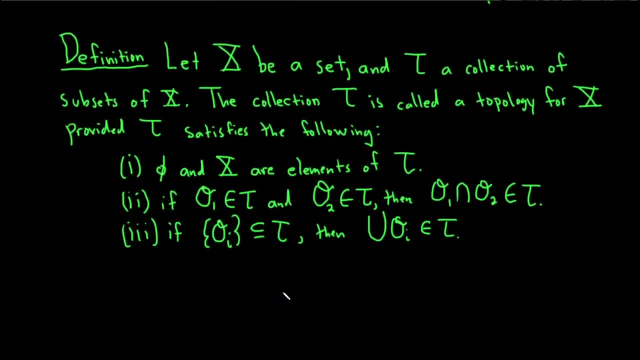 so if we have these three conditions, then we say tau is a topology for x. so again, the empty set and capital x are in tau. if you have two elements in tau, the intersection is in tau, and if you have any number of elements in tau, then the union of those elements is also in tau. 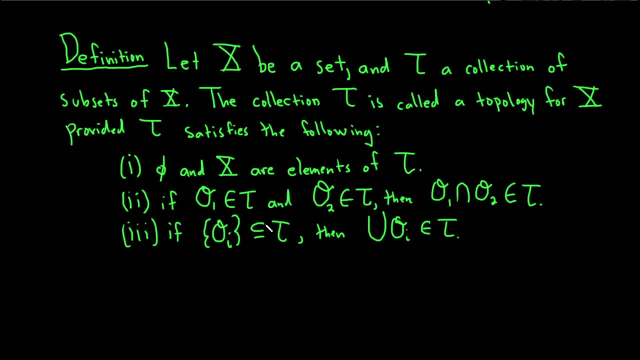 so what is this notion of open? so we define open sets to be the elements of tau. so all of these sets that you see in tau are actually the open sets. so the elements of tau are called open sets. so, so, so, so if you wonder, okay, so what does it mean to be open? well, it depends on tau. it will depend on. 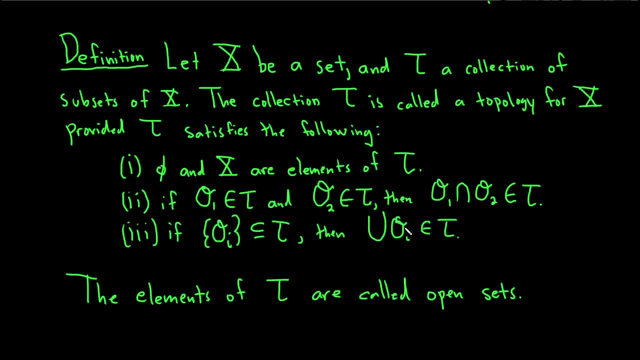 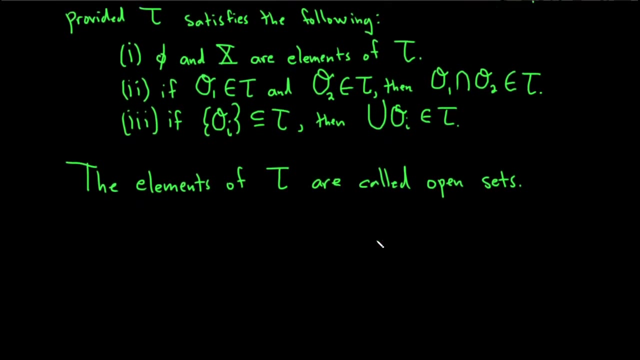 your topology. each topology is different. open sets are defined differently in different topologies, but in general, you know, any element of a topology is called an open set. so that's something i think that sometimes people get a little bit confused. all right, so let's keep going. let's look at some simple examples of of topologies. so let's look at our. 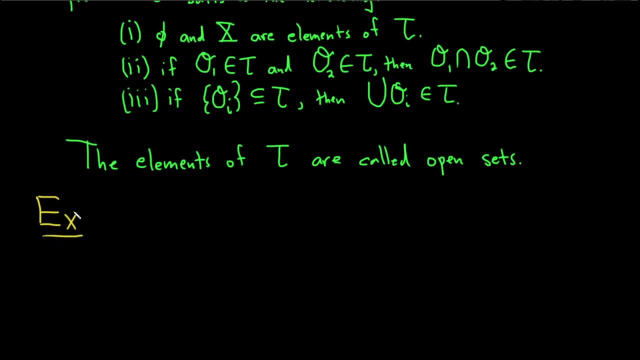 first example here, and let's look at a very simple case: we're going to let x be a set, so it's just some set- and we're going to let p of x. this is going to be the power set. so this is the power, this is the power set of x and what this is. 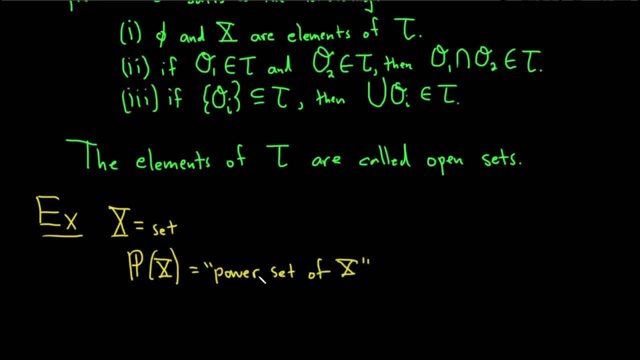 is that we're going to have a set of p of x and so we're going to have a set of p of x. It's the collection of all subsets of X. So this is all subsets of X. So let me just do it here. 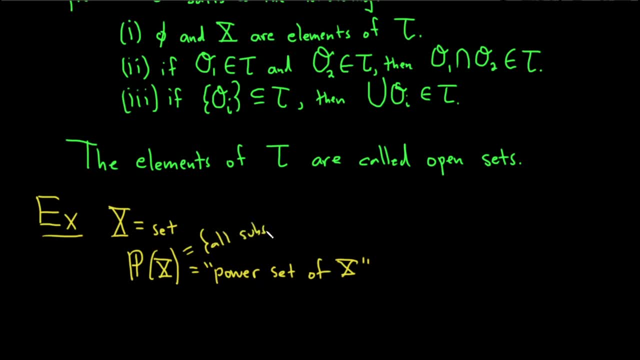 This is all subsets of capital X, Every single one, All of them. And it turns out that this is going to be called the discrete topology. So this collection of subsets is a topology for X. So this is your tau. Your tau is the power set of X. 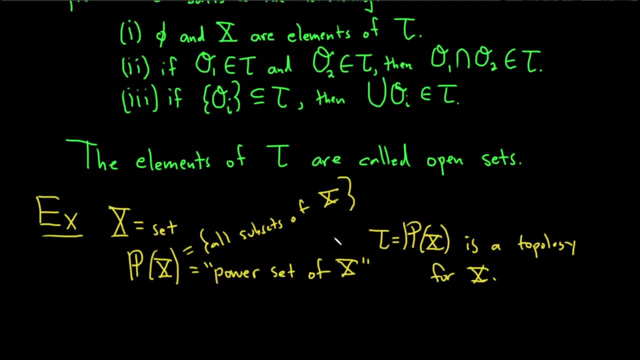 And it's a topology for X because it satisfies all the conditions right, It's all subsets of X. So the empty set and capital X are going to be in here because they're subsets of X. If you take any two subsets of X. 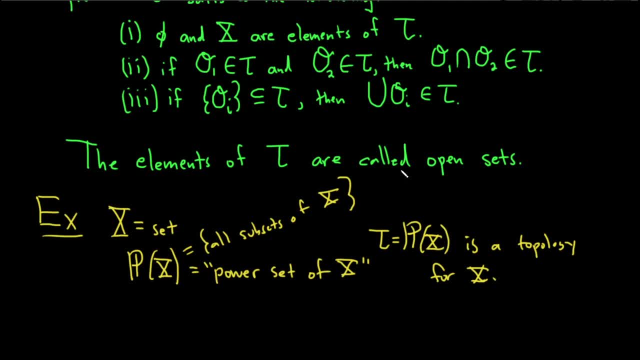 and you intersect them, it's certainly going to be a subset of X And if you take any number of subsets of X, the union of those subsets is also going to be a subset. So it's very easy to see that it is a topology. 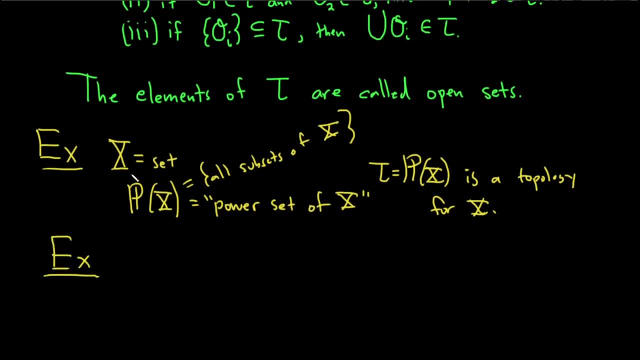 So let's do another example of a topology. So this one's a little bit different. This time we're just going to say X is a set And then tau is going to be a set. So tau is going to be the empty set and capital X. 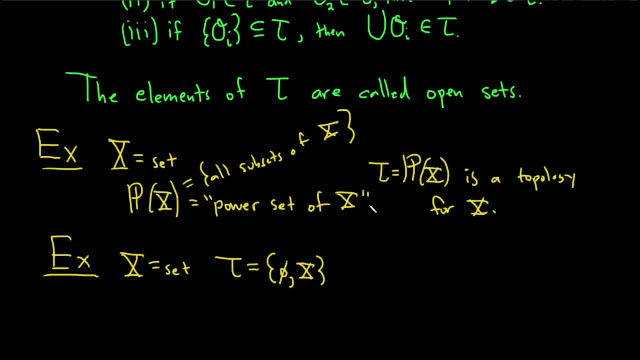 Oh- and, by the way, I didn't write it, but I said it- This one is called the discrete topology. So example one is the discrete topology. All right, so it's topology consisting of all subsets of X. So if you're a subset of X, you're an open set. 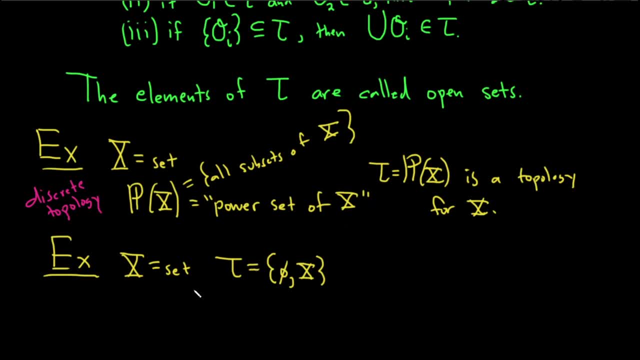 So boom, super easy to memorize. So this one is like the opposite kind of. This one is called the trivial topology, So this is a topology on X And this one is called the trivial topology, So trivial topology, So it's just X is a set. 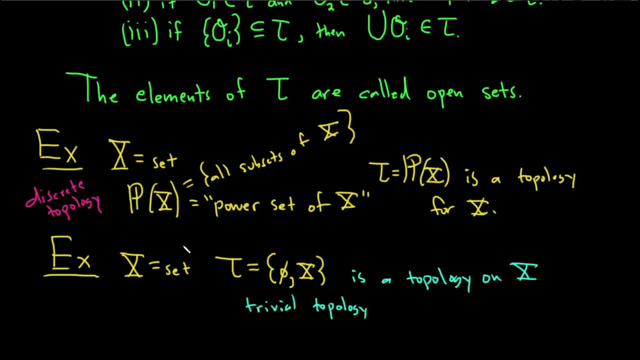 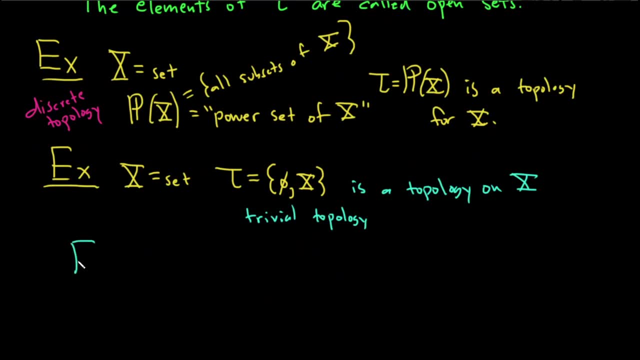 and then you just take: Oh, X is any set, and you take this and you're good, All right. Let's look at another example. How about this one? So X here is a nonempty set. And let's take little A in capital, X. 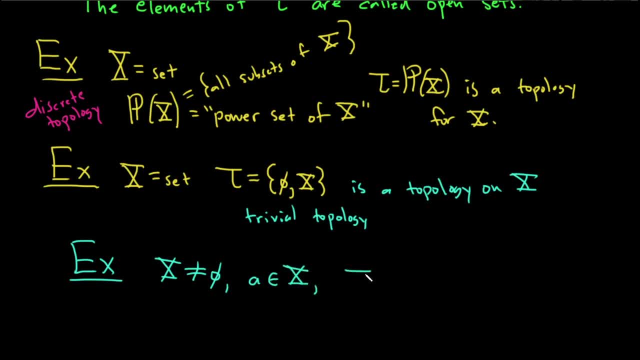 And we're going to define tau as follows. So tau here is going to be the empty set, the singleton set containing A and the entire space, And this is a topology on capital X. So if it contains A, it contains the empty set. 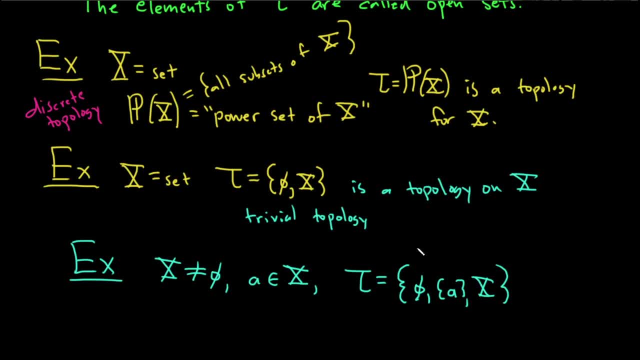 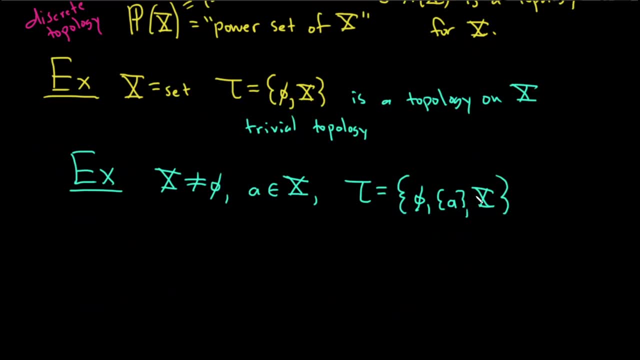 and it contains capital X. So that was the first condition, if you recall, had to contain those two elements. If you intersect any two elements here, you're going to get an element in the set. So you know, empty with empty is going to be empty. 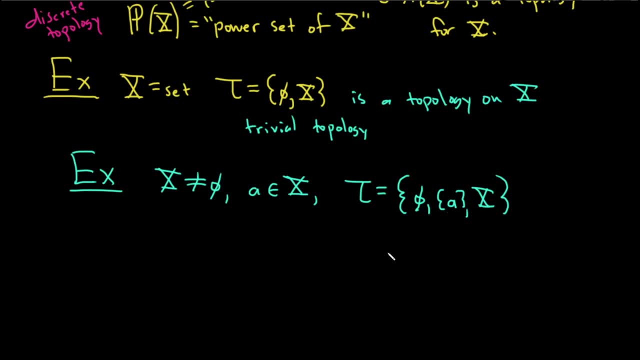 If you intersect the empty set with any of these, it's the empty set. If you do something like this, you're just going to get this, which is still in tau. So any intersection of any two sets in here is in tau. 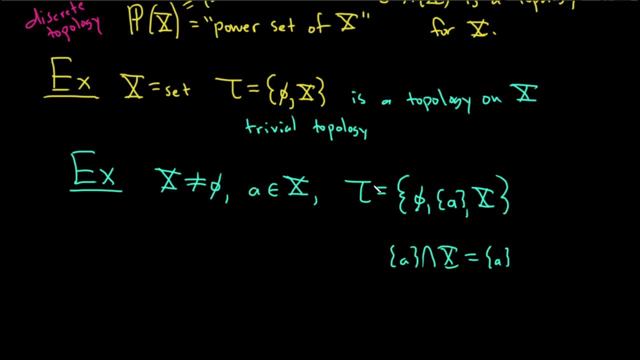 And the union of anything in here is also in tau, So this is certainly going to be a topology. All right, Let's do another one. This is a little bit harder. This one is: X is a set containing the following elements: It's just A, B, C, D. 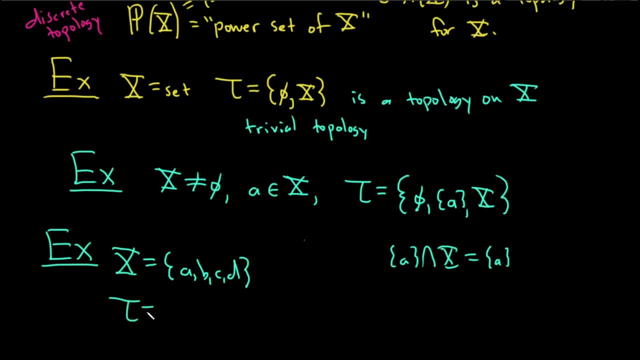 And we're going to say tau is the collection of sets: The singleton set containing A, the set containing A and B, and then the set containing A and C, and then the set containing A, B and C, And of course we still need two more special sets. 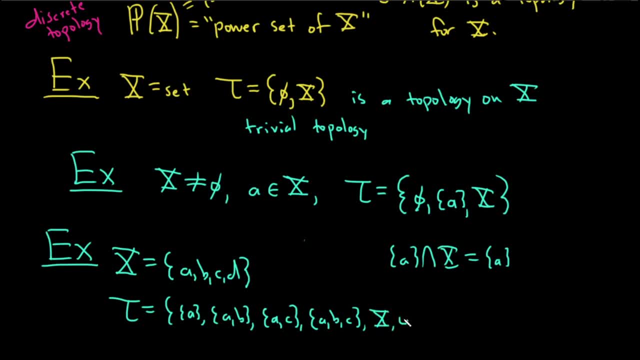 We need the whole space, right, That's the first condition. and the empty sets. We do need both of those, And this is a topology for X as well. So this is a topology for X as well. So this is also a topology for X. 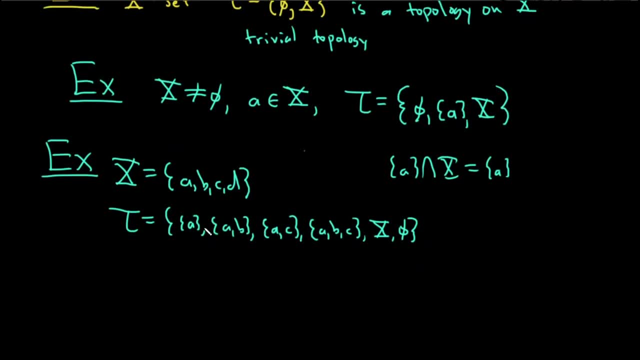 And you can check all three conditions if you want to. You would have to write it out. It would take a lot more work. You could do it mentally, But if you listed it out it would take some time to verify it all.